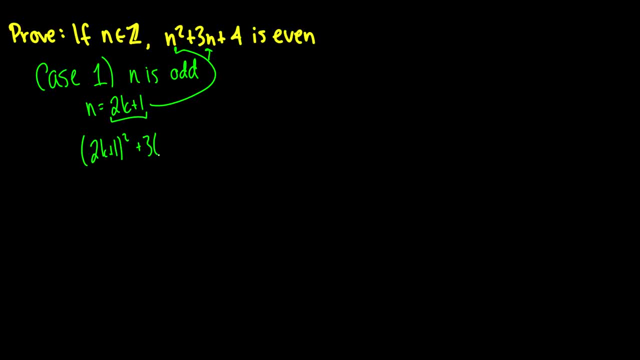 2k plus 1 squared plus 3 times 2k plus 1 plus 4, which is going to be 4k squared plus 4k plus 1 plus 6k plus 3 plus 8.. Then, when we collect all of our terms here, we get 4k squared plus. 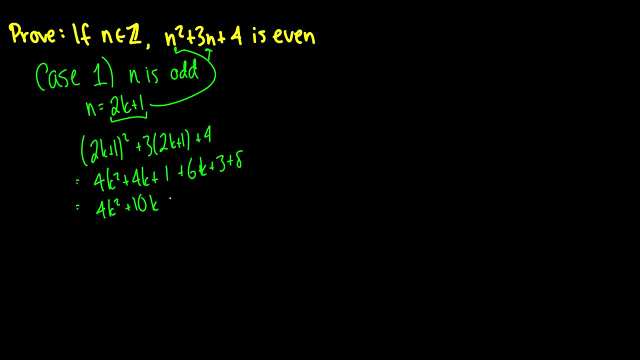 plus 10k plus 12, and all of these terms are divisible by 2,. therefore n is even So, or sorry? then n squared plus 3n plus 4 is even so. that's good. Case 2,: 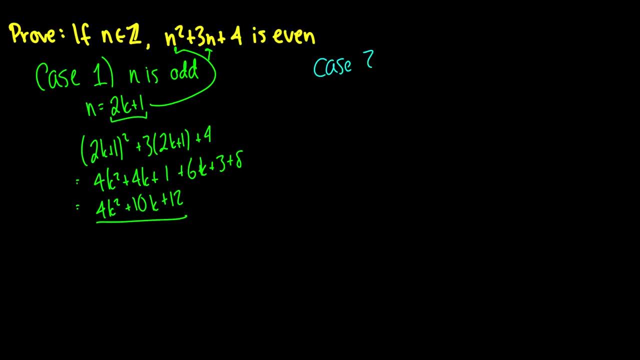 we have to say: okay, well, what if n is even now? So then n is equal to 2k. Well, this should be a little bit easier to solve, at least algebraically. So we have 2k squared plus. 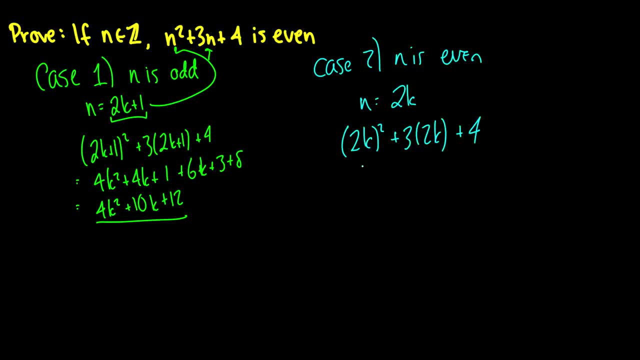 3 times 2k plus 4, which will be 4k squared plus 6k plus 4.. Again, the whole thing is going to be divisible by 2k squared plus 3k plus 4, which is going to be 4k squared plus 6k plus 4.. 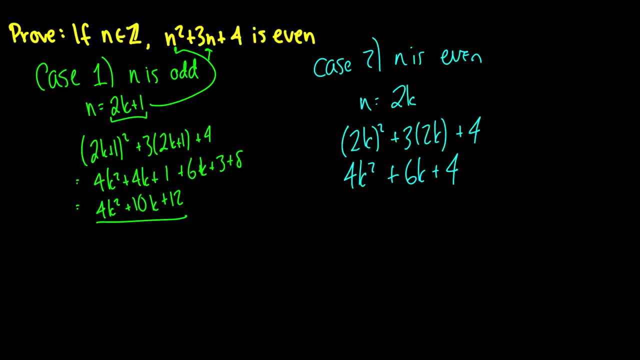 Therefore we know that it is going to be, even if our n is even as well. So because we've proven that both are even independently, both can become even, we can conclude that n squared plus 3n plus 4 is always going to be, even if n is an integer. So that is a very specific. example of how we can solve this problem. So we have 2k squared plus 3n plus 4, which is going to be 7.. So we have 2k squared plus 3n plus 4.. So that is very specific example of a proof-by-case. 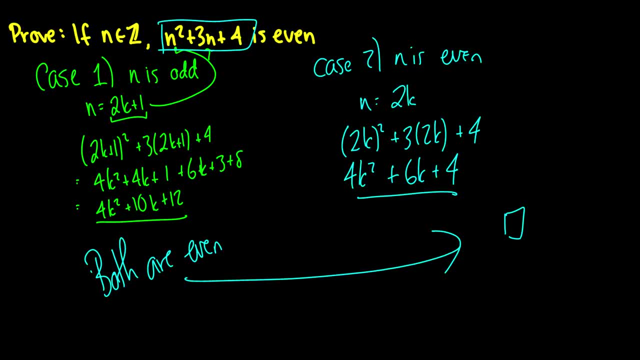 Honestly, there isn't much more to that. Proof-by-case is just a technique that has to be used in some proof. It's not really a method of choosing how to prove something. It's more like: depending on how you choose to prove something, you may or may not need to use proof-by-case. 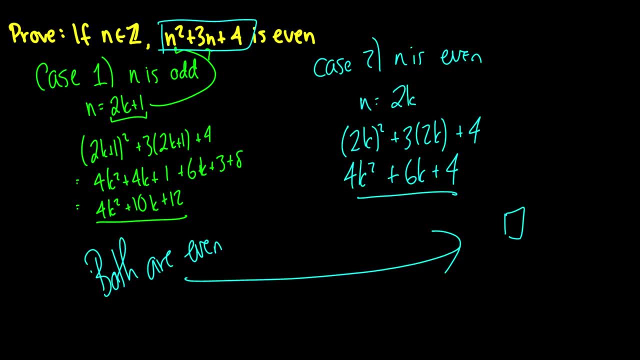 So that is why this video is incredibly short, because it is a tool that sort of tags along a bunch of different tools you could select. It's either required or isn't, So that's Root by Case. If you have any questions, leave them in the comments below and I will get to you. as soon as possible.